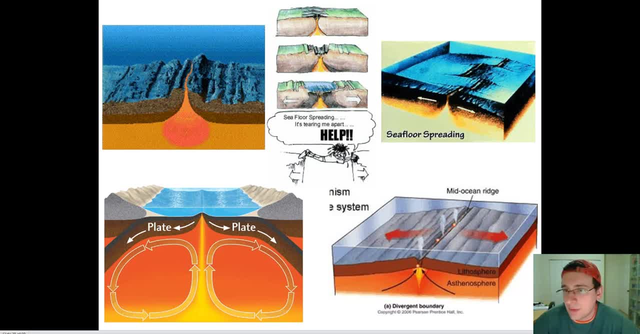 And until the 1940s or the middle of the 20th century we didn't really know what this missed mechanism was. But once we started using sonars and water to find submarines and things- ships under the water, we soon realized that the shape of the bottom of the ocean was actually very intriguing. 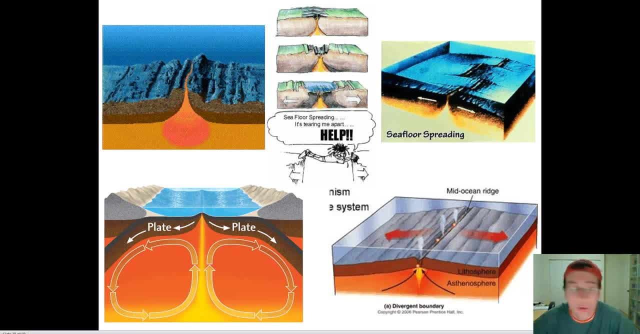 And we started finding things like seamounts, guillots and the mid-ocean ridge in the middle of the ocean, And as soon as people realized that there was this mid-ocean ridge in the middle of the ocean, questions were raised about what that was and what was the role of that in the Earth's system. 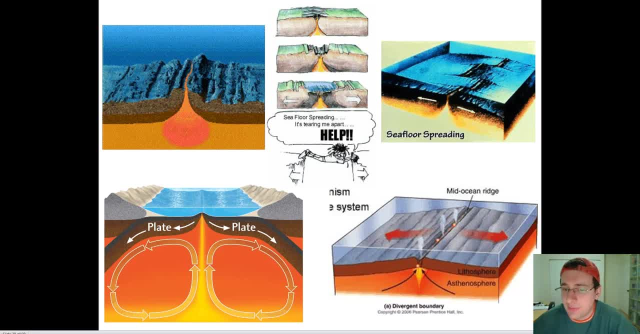 And so oceanography research became the geological evidence that ended up proving Wofford Waggoner's continental drift theory. The idea of seafloor spreading, or the idea that magma rises from the inner core through the mantle, pushes through the crust of the Earth and eventually creates new crusts that push the continents apart, is actually the missing mechanism that Waggoner was looking for to explain how the continents could possibly drift apart. 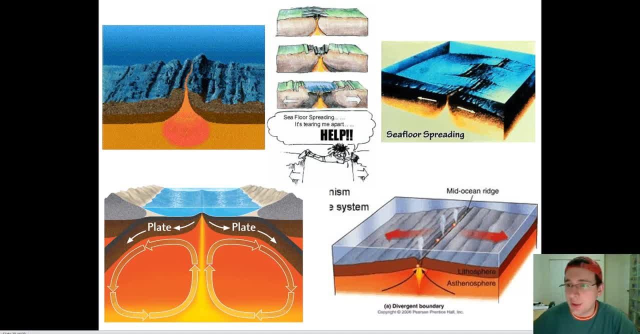 And you actually see this process shown here on the screen In the middle. there you see the guy trying to hang for his life as the continents are drifting apart- And certainly this was the case for many animals when this first started happening, because this actually separated animals that live in different continents. 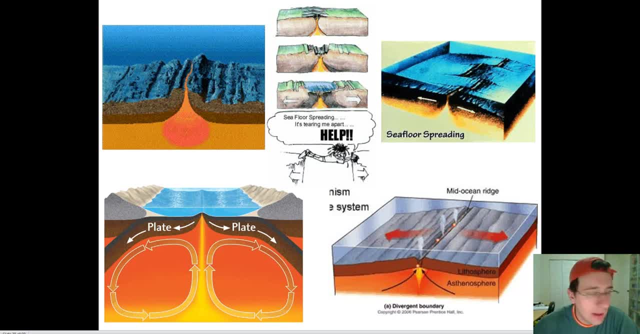 And this explains why we find fossils across different continents. They may have been dead for a long time or they may have been actually alive in the time. the continents are actually trying to separate from each other, But the way this will look like basically is that magma from the inner core is going to start to punch through and try to find the easiest spot to punch through. 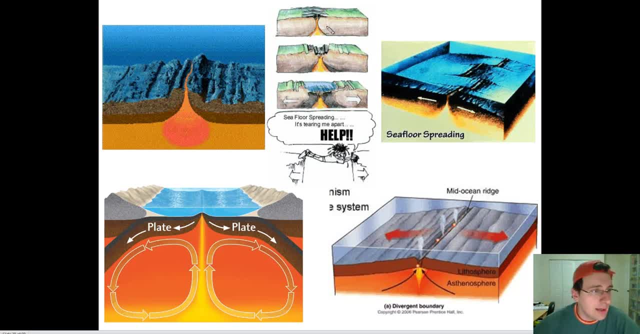 It will find a fault line, rise to this fault line, punch through it and eventually melt the surface of the Earth and the crust and eventually cause the crust to bend upwards like this, And when it gets thin enough, it would actually rip the crust apart. 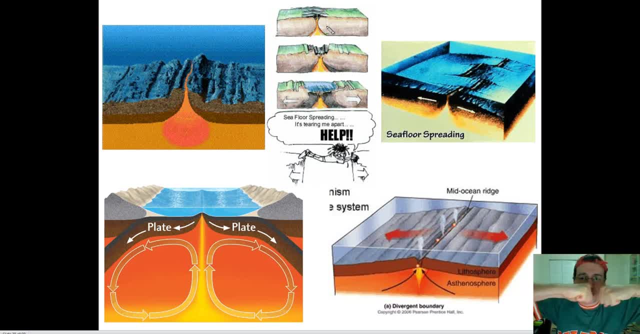 So what I want you to imagine is a piece of paper that's been stretched and stretched and stretched and stretched, bent up, bent upwards, until it eventually cracks. And that's what happened to the surface of the Earth. But when the surface of the Earth cracked, magma seeped through and sealed that crack with new crust that immediately solidified. 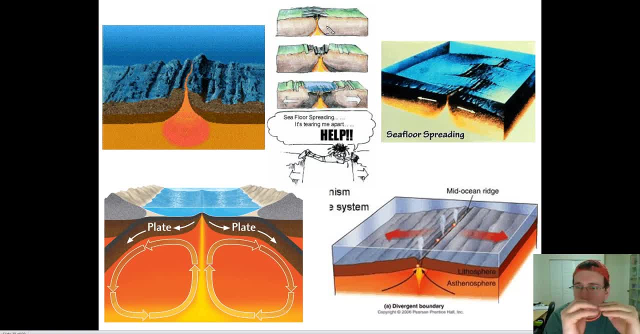 But that new crust was very flimsy and probably the thinnest part of the entire crust, So that's the easiest spot for the magma to come through. So that's the easiest spot for the magma to come through. So that's the easiest spot for the magma to come through. 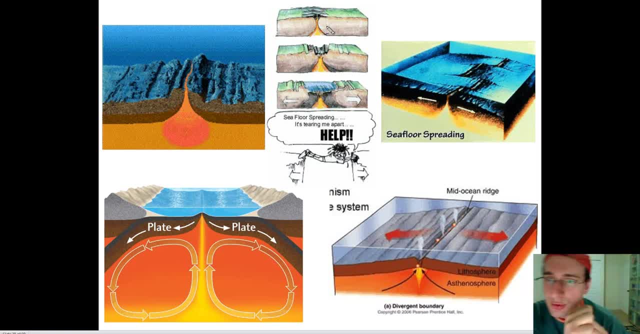 And that's the easiest spot for the magma to punch through again. And so again, the magma was going to punch through that crust Again. it creates a gap, pushes the crust apart a little more, seals the gap as it solidifies. 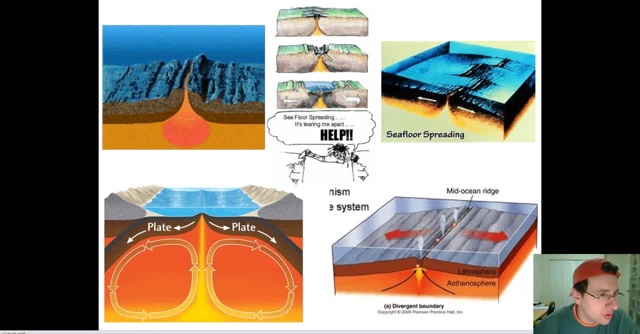 And as the process repeats over and over again, push after push, you're going to create these fractures at the edge of the actual zone that's being cracked and pushed. But as new and new magma actually fits in between, you end up pushing the contents apart from each other, and then oceans will float. 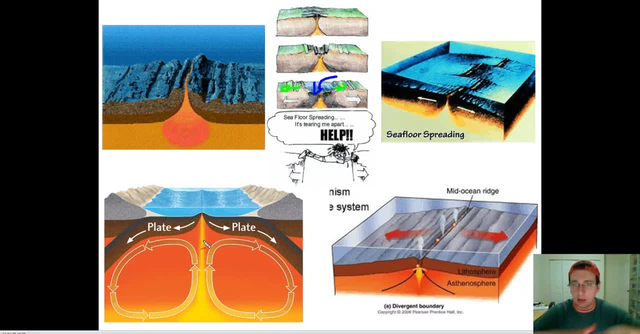 And eventually, over a period of millions of years or so, you'll get something that looks like this: The mid-ocean ridge will still be in between, The magma will still be lifting the middle up, It will still be fracturing that middle, still pushing it apart as it tries to fit in between. 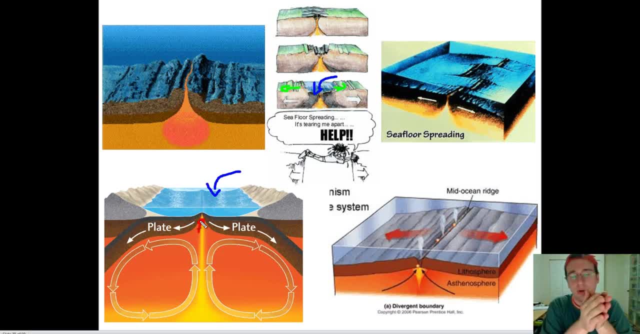 And it will still be creating new crusts, which is the flimsiest of the crusts, which is the easiest way to crack again And be pushed to the side again. And over thousands and thousands and thousands of years, you're going to create new and new bands which will flow away from the middle. 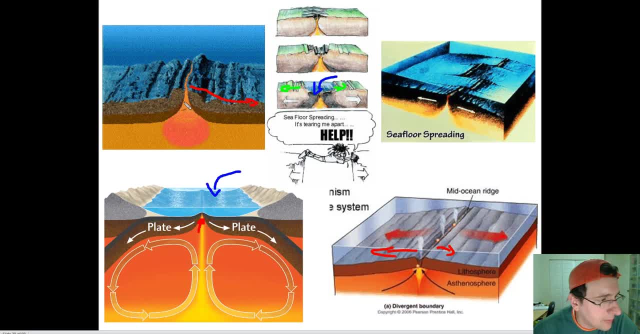 And as you are pushing it away, you're going to go further and further from the area that's being bent upwards and become flatter and flatter ground. as the folds are stretched thinner and thinner and the seafloor is created Later, the actual crack can actually shift and different pieces of the crack can be bent in different directions. 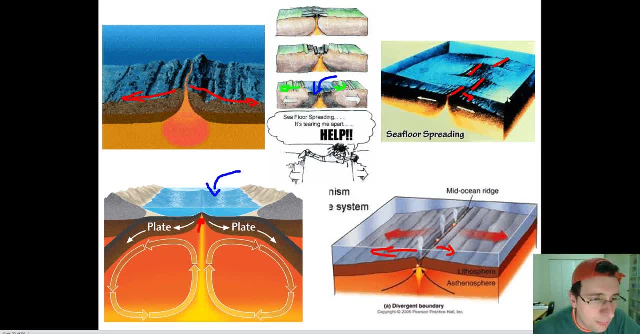 So, for example, maybe this piece here, This piece here, moved more this way and this piece moved even faster, This piece moved a little slower, This piece moved faster And what you get is that the actual mid-ocean ridge not 100% aligned, but like different pieces of it shift to the side and transform boundaries. 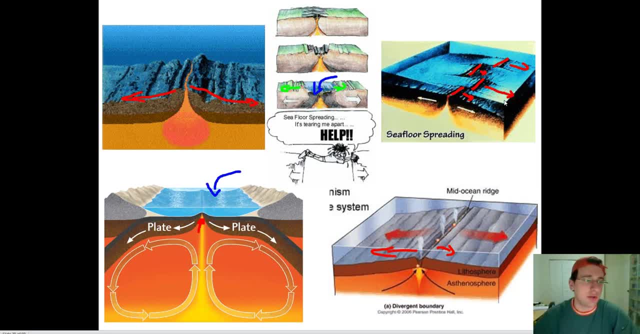 And the whole thing, though, is full of fractures, and we call that a fracture zone- And this process of seafloor spreading, of the magma rising, becoming lava as it touched the surface, By the way. that's the difference. 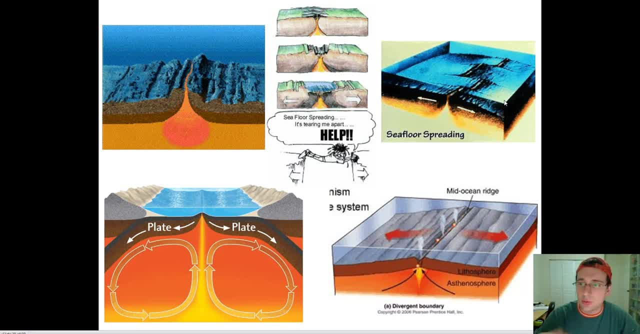 That's the difference between magma and lava. Remember, magma is underground, Lava is, when it reaches the crust, all right, And it becomes exposed to either the air or the water. And so when this lava solidifies, makes new rock, pushes the crust apart, it's flimsy cracks again. 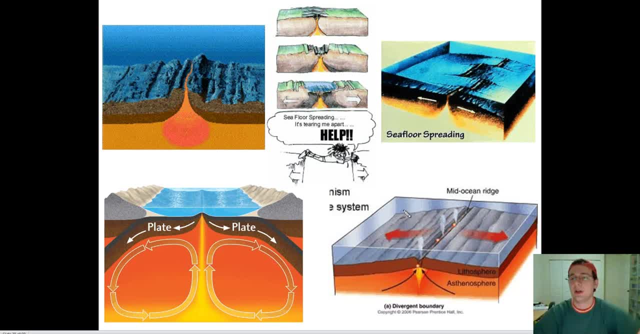 Lava pushes through, pushes the crust apart, solidifies new crust, And so this process starts over and over again and ends up creating the separation between the continents. All right, Now what evidence is there to support that this is actually a fact? 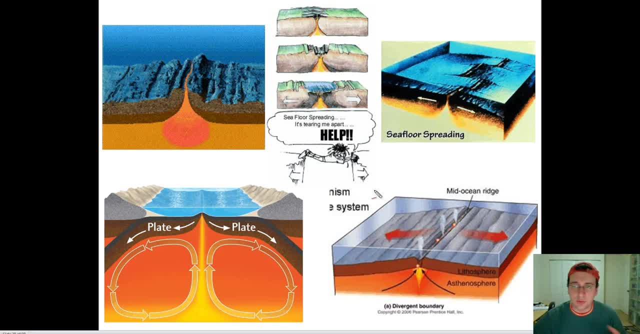 That we actually have seafloor spreading, Because when you look at the mid-ocean ridge, all you see is a ridge. You don't actually see this happening. You can't actually quantify this happening, at least not until very recently. So what evidence is there to figure out that this is actually indeed happening? 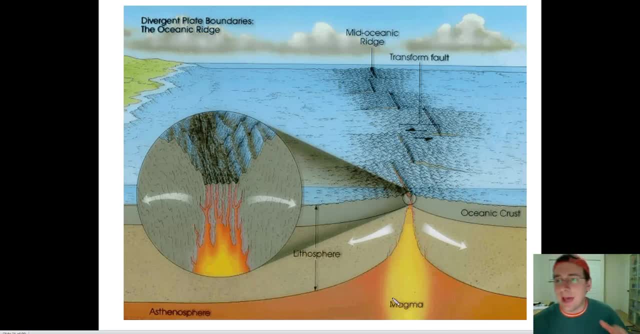 Well, remember, the rift itself is evidence that something is happening here. If you look at the rift and study the rift- we did that with robotic submarines and things like that- We noticed that there's actually a large, large valley in between two large mountain ridges. 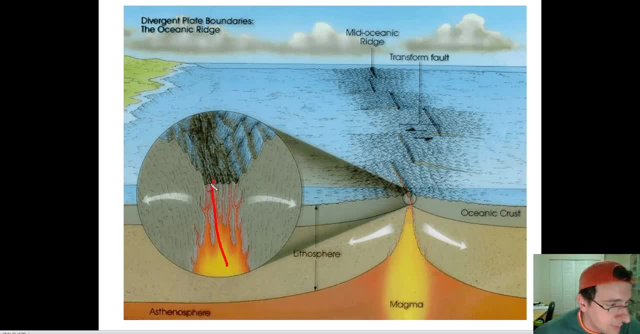 And that in that valley, you have cracks in the surface of the earth where magma is seeping through to the surface And as it does this, it pushes through the surface and pushes the crust apart. Now, as you can see here, each one of these bands that you see here is one event of a crust being created. 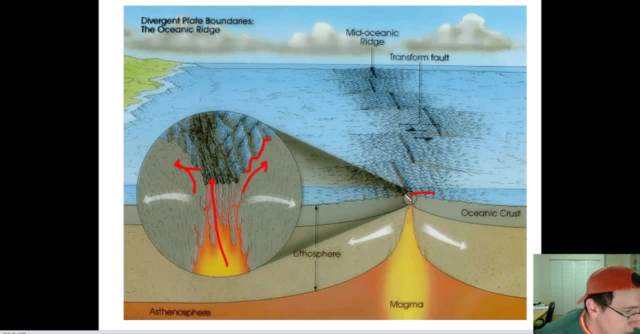 And as the crust is being created away from this region, it starts to travel more and more away from the mid-ocean ridge over a long period of time And eventually it's gone. It's going to travel away from the area that's being pushed up and cracking and form the large abyss. that's kind of flat, especially as this stretches away. 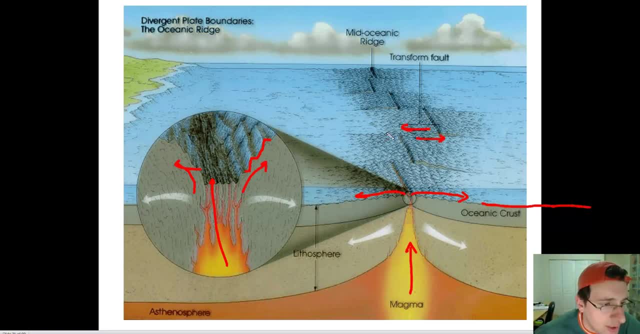 Also remember that you could have a transform fault where one piece is actually moving to the side in relationship to the other piece because of the way the magma is moving underneath that fault line, But that overall you get in the middle of the entire ocean basin a pattern of cracks, one next to each other. 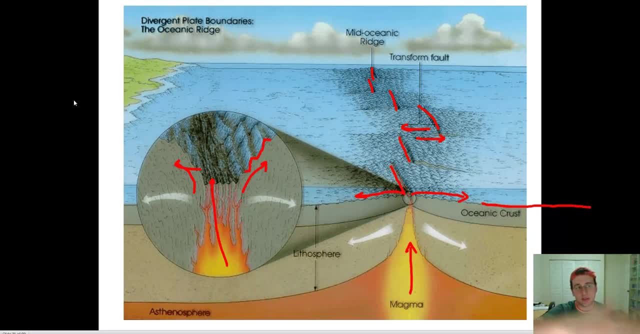 Not necessarily lined up with each other, but one next to each other across the entire middle of the ocean, And that's what's actually spreading the ocean, And this is the perfect example of a divergent boundary. When we talk about this again, remember this picture. 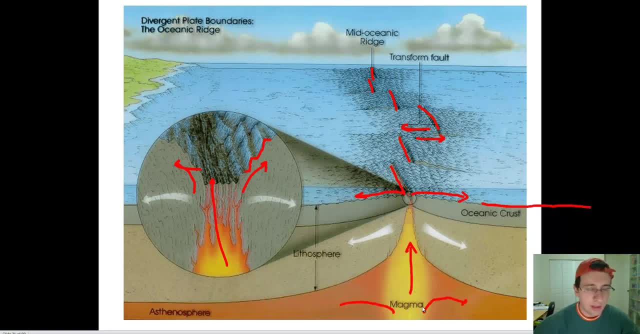 It's a good picture to study and see how a divergent boundary looks like. Remember that this is happening because the lava is flowing. magma is flowing away from this central location, dragging the asthenosphere to the sides, this way away from each other.